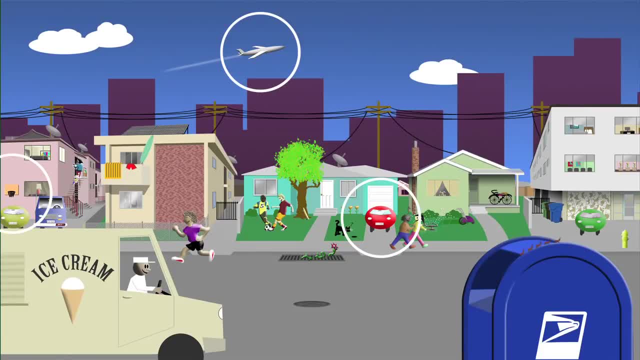 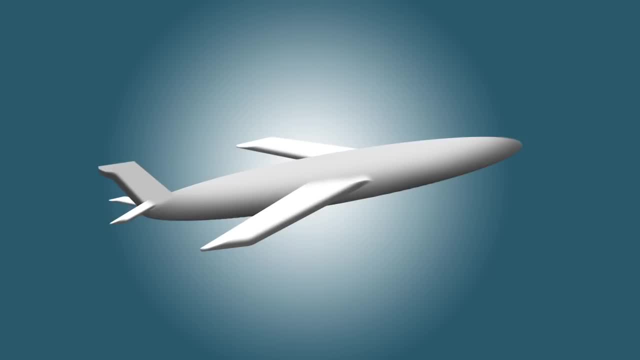 The car in the driveway and the basketball hoop on the building. I think of what makes a car go, what gives it its propulsion, By what means does it go forward? The airplane in the same way. it's going through a different medium. 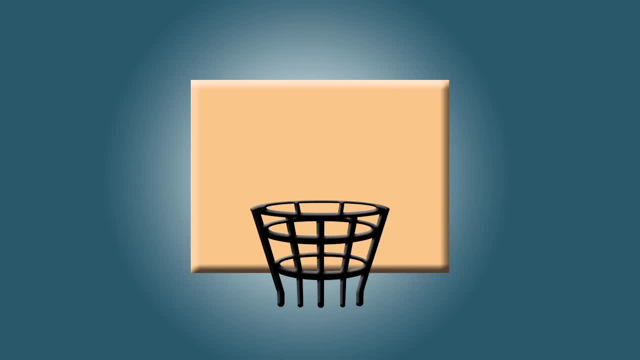 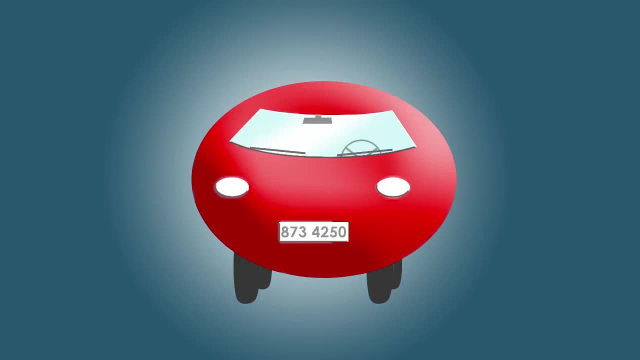 So how does it achieve that With the basketball hoop? one thing that would be pretty neat is to make all your shots every time. Well, why not build a robot to do the job for you? There's a lot of ways to improve things. 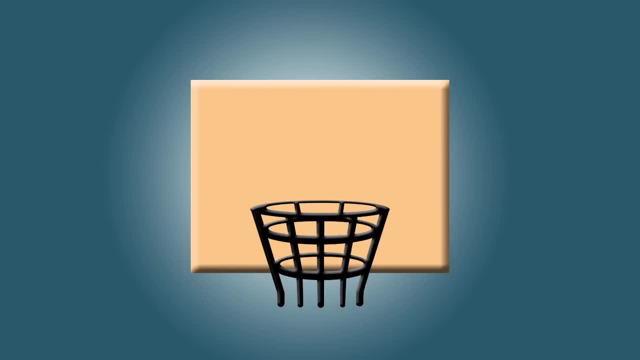 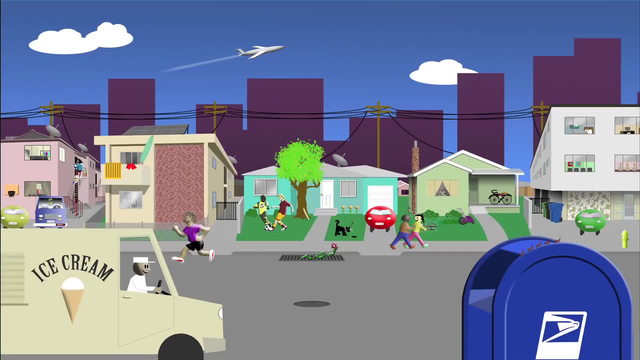 You can make a car go faster, a plane fly farther and make every free throw. Okay, so you have several ideas You could then develop perhaps into a question. Serena, do you see anything you could ask a science question about? I see the plant growing out of the drain and it leads to questions about how do plants grow? 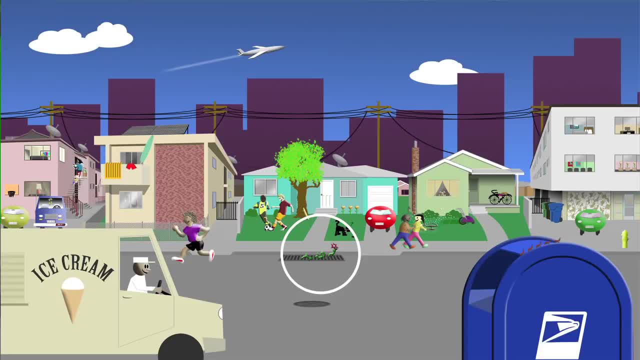 What sort of conditions do they grow best under, For instance, how much soil do they need or different types of fertilizer? I see the person running and I'm a runner myself, and there's a lot of experiments I do just on my own. 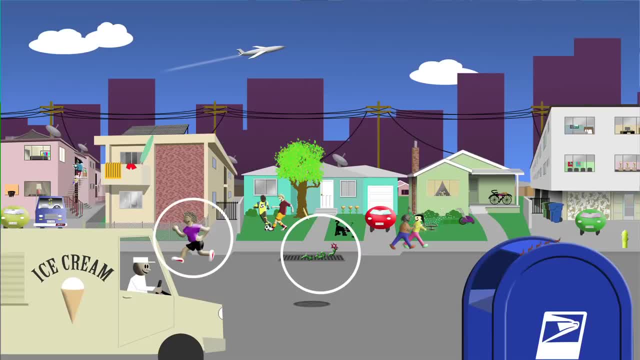 in terms of how much water do I need, how much rest do I need, what's the best way to recover after a run That leads to possible results? I see a lot of scientific experiments And then, finally, I look at the windows and I wonder: what are the best types of covers for keeping a house cool? 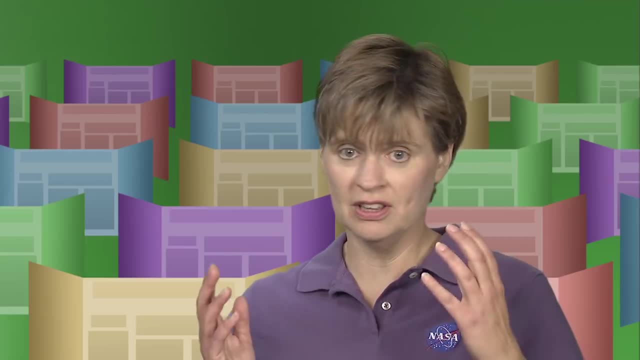 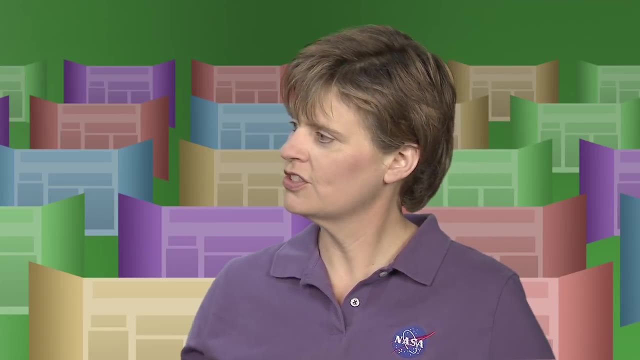 All right, so you both gave me about three ideas. just glancing at this image. If I gave you more time, do you think there are more things you could see or come up with from this image? Infinitely many, Infinitely many. 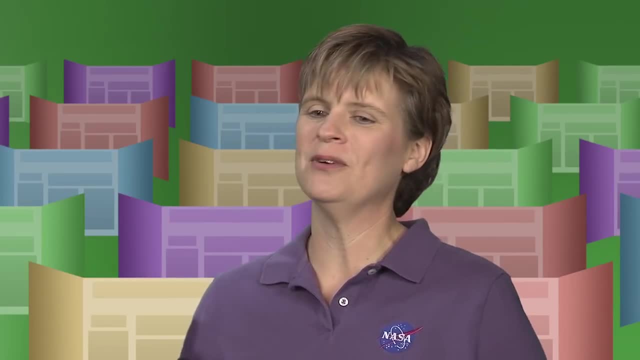 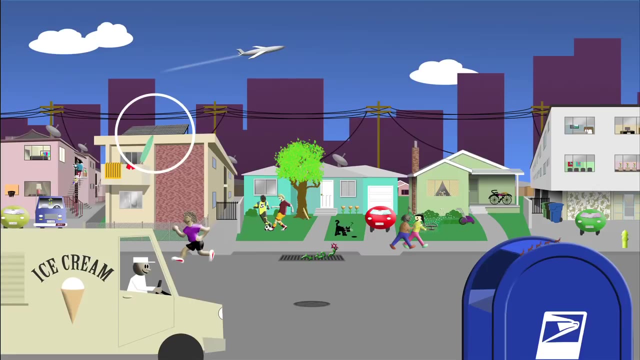 Absolutely Okay. I'm going to prod you to give me one or two more that you have an idea of. If I was a little kid instead of a big kid, I'd be really curious to see what those things would look like. What are those things on the roof of my family's houses? 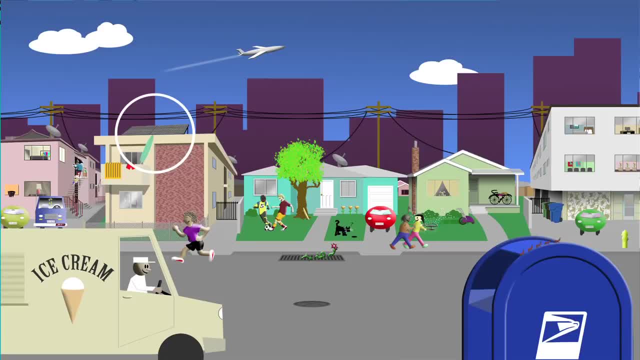 How do they work? You're turning sunlight into energy. There must be some interesting things going on in there. Someone who likes sports? you've got different ball shapes. Maybe they all move differently through the air when you throw them. You can look at different designs there. 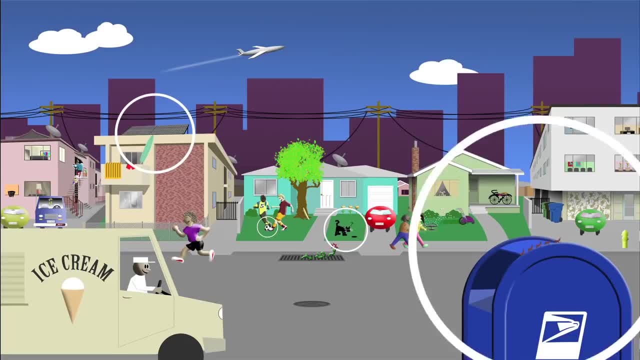 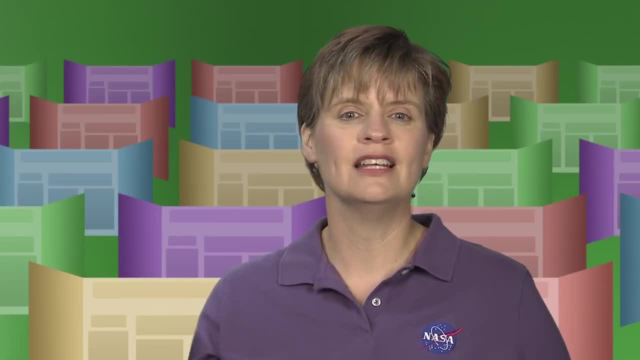 There's a cat. You can ask questions about animals. There's the bugs. What type of food do ants prefer? There's lots of things in this picture. Ask questions about whatever you can see. Look around, open your eyes and view things in a different way than you ever have before. 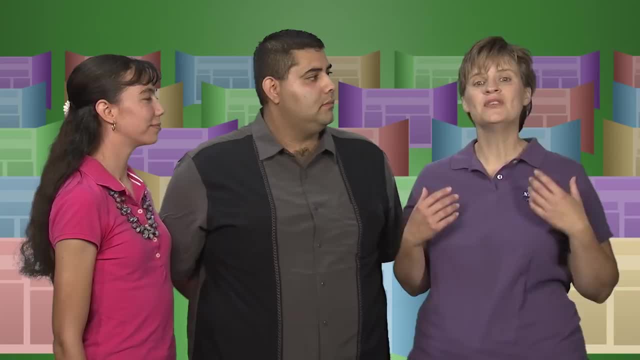 Up. next, we will help you develop your observations into testable questions.